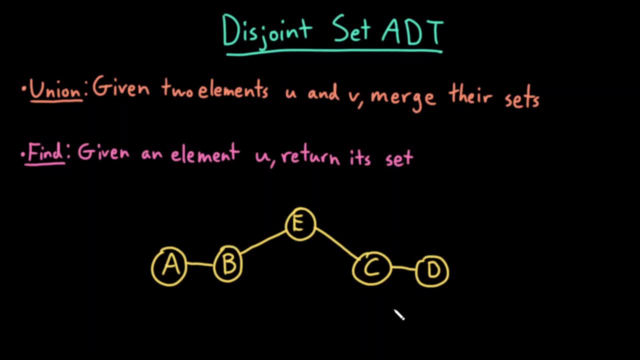 that joins these two transmission clusters and merges them. So in reality, we now suspect: oh uh-oh, there's probably a single large transmission cluster from which all of these people came. Let's think about that operation. Basically, we have to have some way of representing individuals. 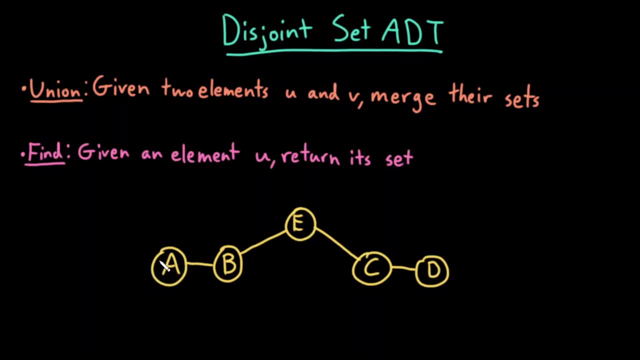 and we have to have some way of representing- or how can we actually figure out- what cluster each person is from, And we have to have a way of efficiently merging two different clusters. So, for example, I merged E's cluster, which was originally just itself, with B's cluster and I merged E's cluster. 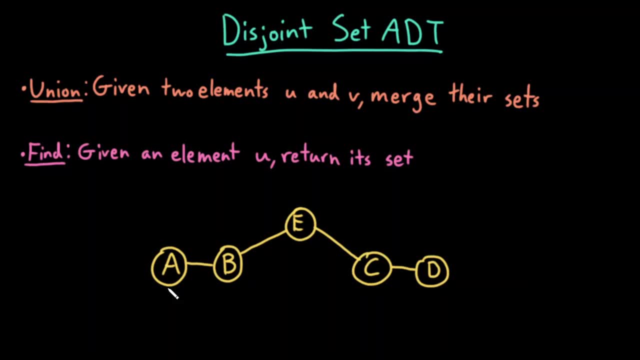 with C's cluster and the result was that this cluster merged with this and then this cluster merged with this, yielding one large cluster. Let's formalize this into an abstract data type. We've essentially defined the following two operations: First, we've defined union Given. 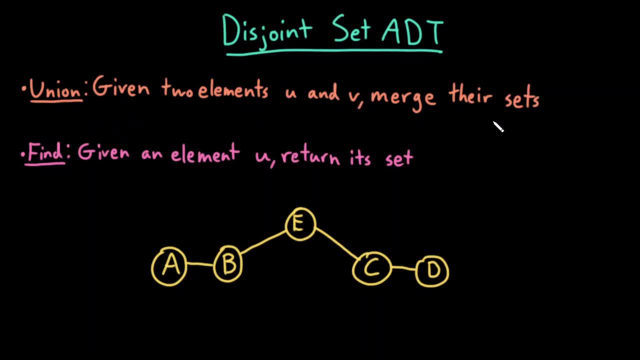 two elements, E and B. merge the sets in which they belong, Merge their sets, right. So if you gave me E and B, I merged their sets. E was in its own set, B was in this set and then I merged those two sets. I performed a union operation on E and B And then afterwards, 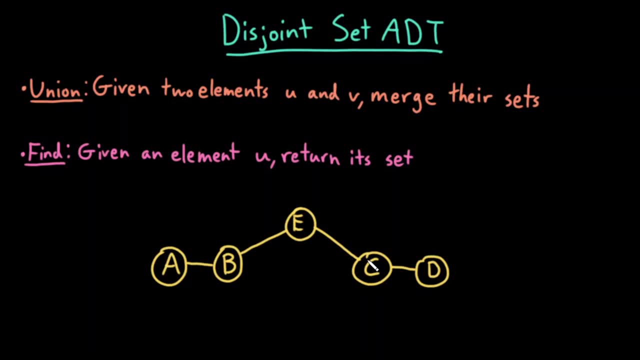 I found out that E and C were closely related. So I performed a union operation on the set containing E and the set containing C. So I performed union on E and C. The second operation would be find. If you gave me an element, 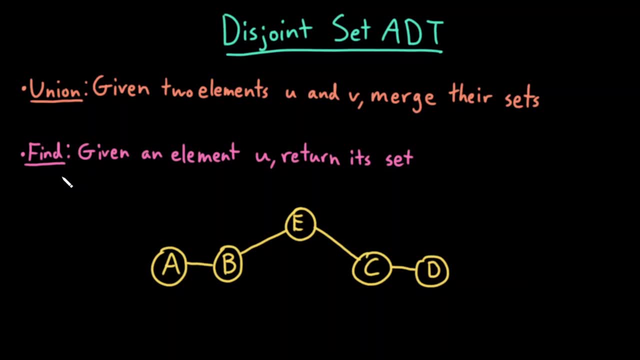 what set does it belong to? This is helpful if I want to be able to identify which individual transmission clusters each person in my community is in. Now, in this simple example, all five are in the exact same set, but theoretically I could have some. 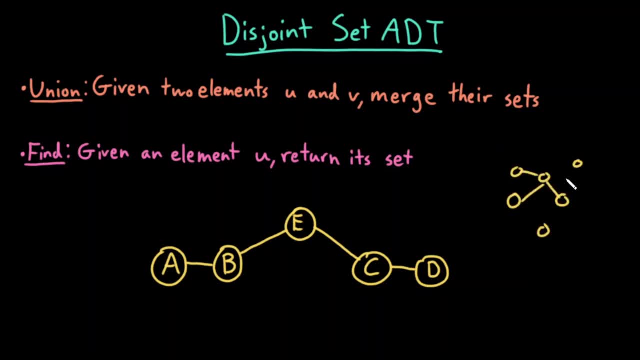 larger epidemic where maybe I have this structure, maybe I have this structure and I have this structure. I might want to be able to identify, given some person, what set do they belong to? This is the disjoint set: abstract data type.